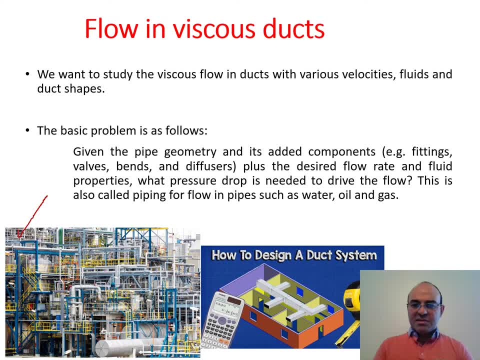 Such as the bands, different kind of connections, diffusers, valves, fittings, and so on are given. Plus the desired flow rate. So, what should be the flow rate and fluid properties. And based on that, what is the pressure drop needed to drive the flow, for instance, in this pipeline. This is a very complex one. Of course, we are not going to study this in this course. Usually, computer packages. 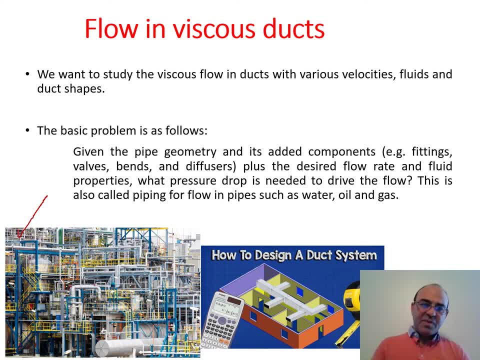 Are used for design and analysis of such complex networks of pipes. However, it is important to know what is in the background of these codes. 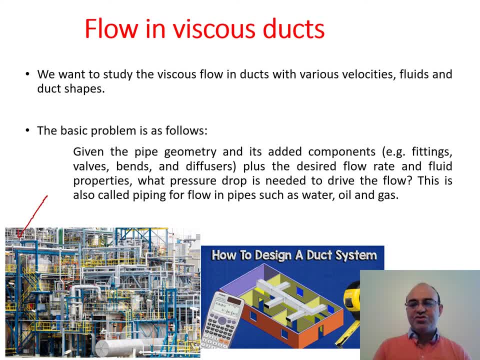 And what is the basic, you know, equations used to design like a pipe flow or duct flow. And this is on the right side. Here you see air duct. For instance, used in heating, ventilation, and air conditioning. 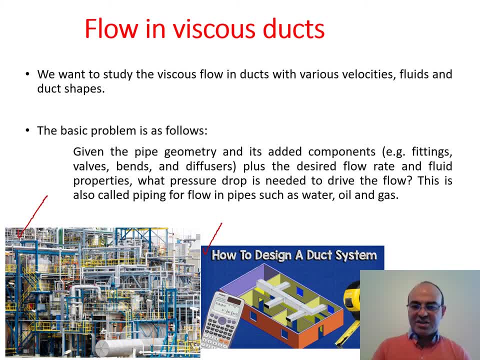 So, similar principles. Here the cross section of this duct is not round. And the fluid is air. 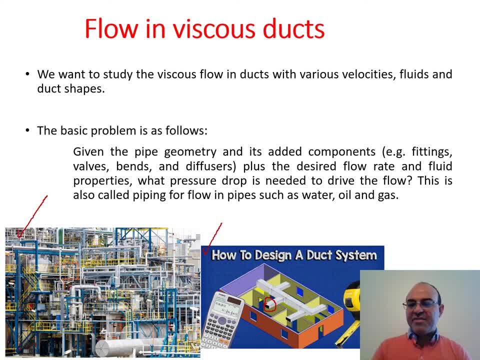 Instead of a pump, here a fan is used or a blower. So, but the principles are pretty much the same. So, in this. So, when we finish this chapter. 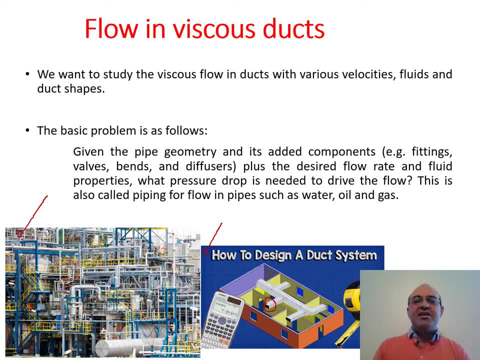 You will actually. You should have like the understanding and skills and some knowledge about how to design such systems. 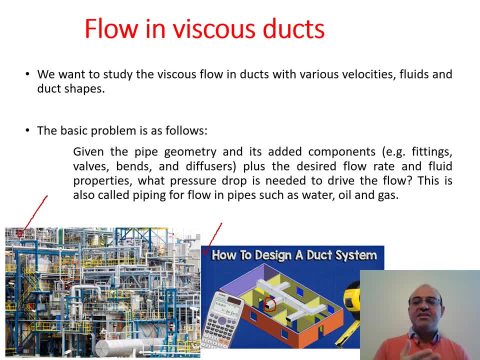 At least, you know, not a very complex network. But like at least on a straight pipe or a pipe with multiple bends. And also with a pump. 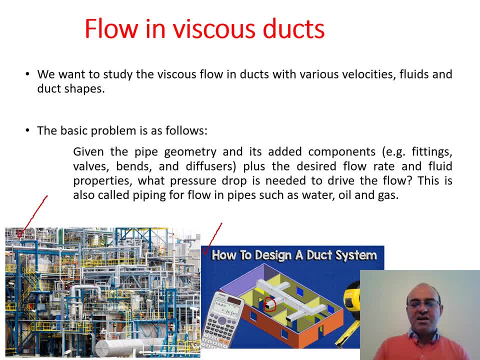 And you should be able to calculate the friction loss. And the pressure dropping the pipe and so on. 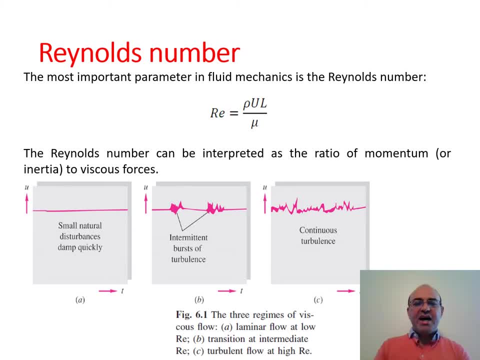 So, let's go back a little bit as a refresher. So, we had in previous chapter the definition of Reynolds number. Reynolds number is in fluid mechanics is the most important non-dimensional number. It is density, velocity, and characteristic length. For a pipe, the characteristic length is. The diameter, usually the diameter, not the length. So, we show it. 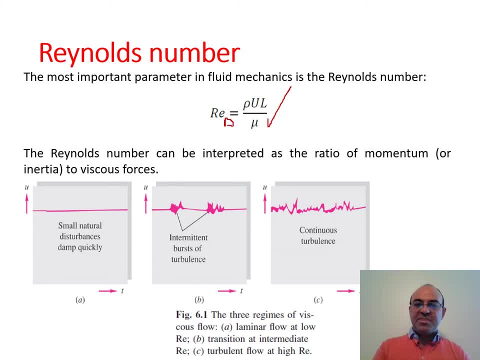 If we show it as Reynolds D. Then it means that this L is equal to D. So, density, velocity of the fluid. Density of the fluid. Characteristic length diameter divided by the viscosity of the fluid. So, it is the ratio. It's interpreted as the ratio of momentum. Or inertia of the fluid. Or the viscous forces. 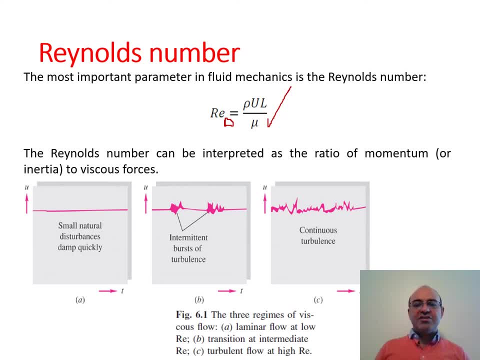 So, it means that the larger the Reynolds number. 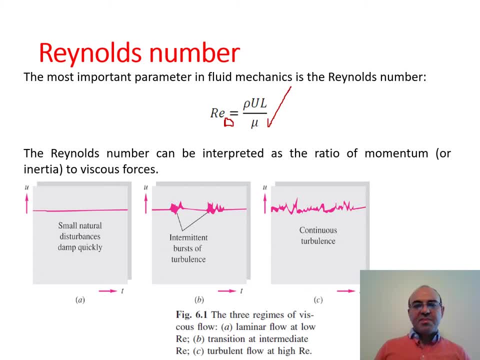 The smaller. For instance, the viscosity. 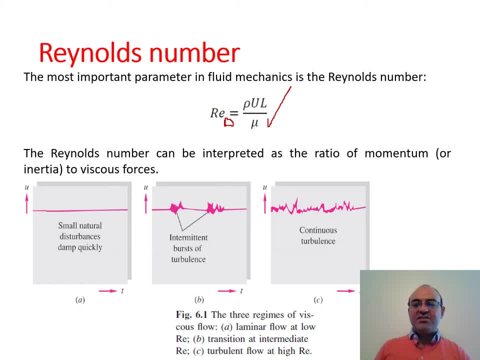 So, if the Reynolds number is large. Then the ratio of momentum over viscous forces is more important. So, viscous forces become like less and less. Less significant. With an increase in the Reynolds number. This is what it means. 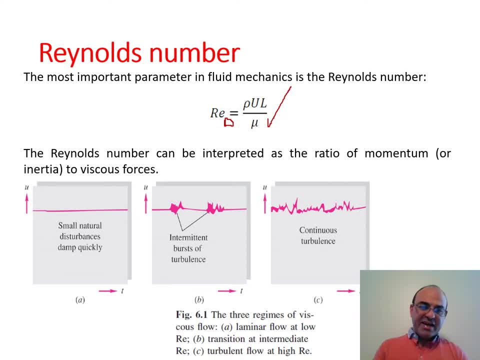 So, if you look at this diagram here. On the left side, we do have a laminar flow. This is like velocity fluctuations versus time. So, the velocity does not fluctuate. So, it's a laminar flow. So, small natural disturbances, even if happen, they damp quickly. If it is very small disturbance. For instance, if you have a laminar flow, you disturb it. It will damp quickly. 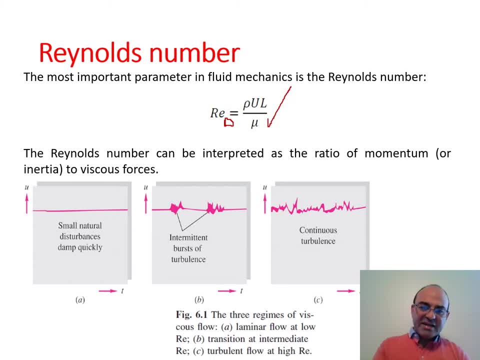 It will not grow. Then as, for instance, the velocity and Reynolds number increases. 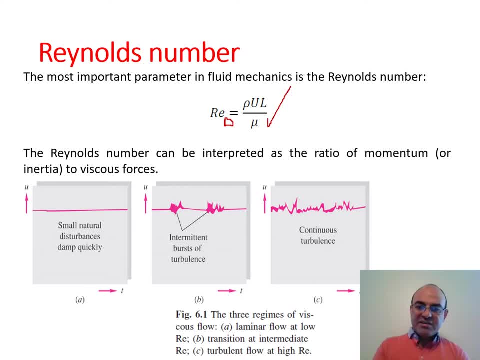 Then we do see some intermittent bursts of turbulence. So, these disturbances appear, disappear. They are there. They are not there. That's called, it is called like a transition from laminar to fully turbulent. 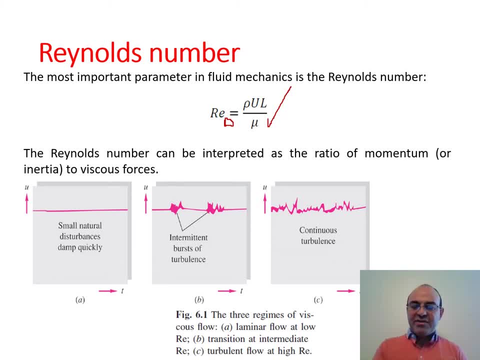 So, in the. Continuous turbulent flow. 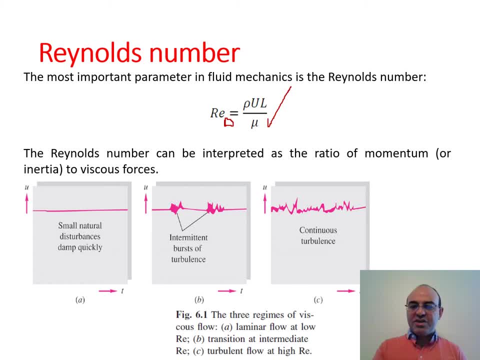 There is significant and noticeable fluctuations. In the velocity components. 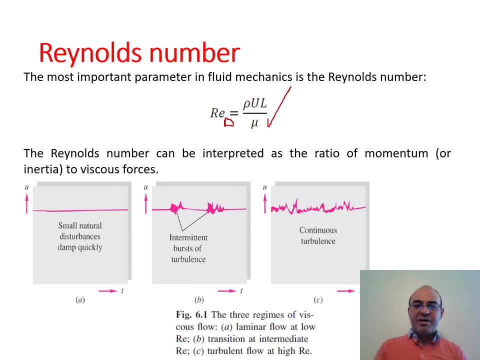 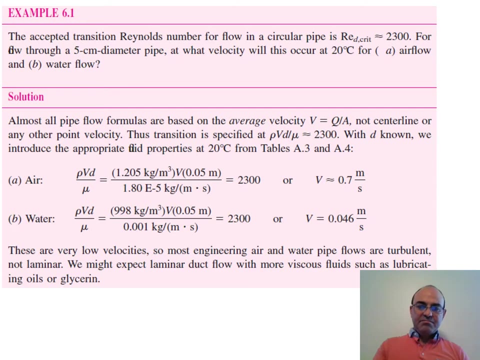 As the fluid flows in the pipe or duct. So, therefore, we do have a region of laminar flow. Trans, transition or intermittent flow. And fully turbulent flow. In the previous chapter, we briefly discussed the fluid in a pipe. 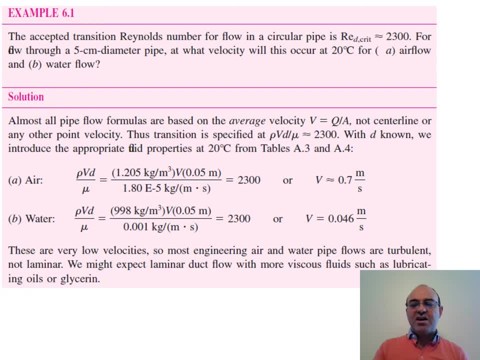 And we said that if Reynolds number based on the diameter of the pipe is less than 2100. Then the flow is laminar. 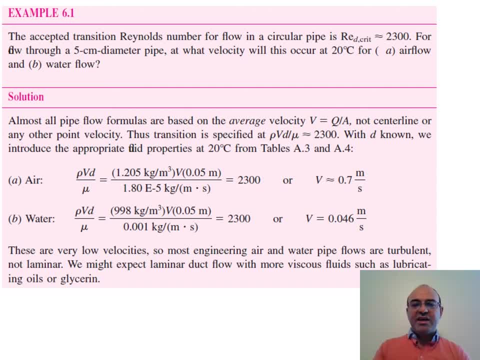 If it's larger than 4000, it is fully turbulent. 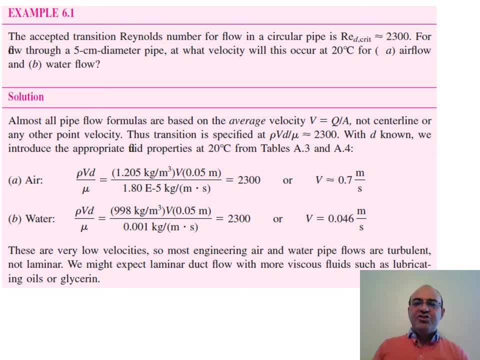 And as a like borderline. Usually a Reynolds number of 2300 is considered. 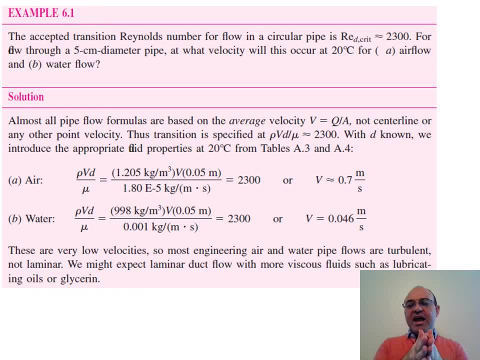 As the borderline between laminar. And then turbulent. 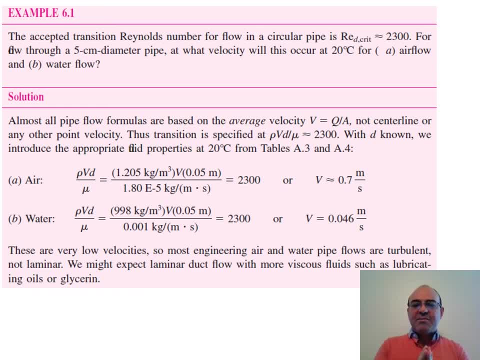 Because usually there. It is difficult to come up with. Or develop equations. For the transition region. As a result. For practical purposes. 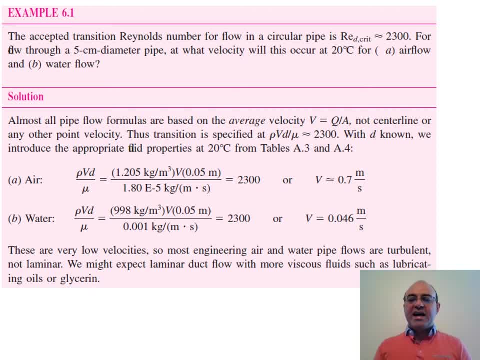 The flow is either considered as laminar or turbulent. 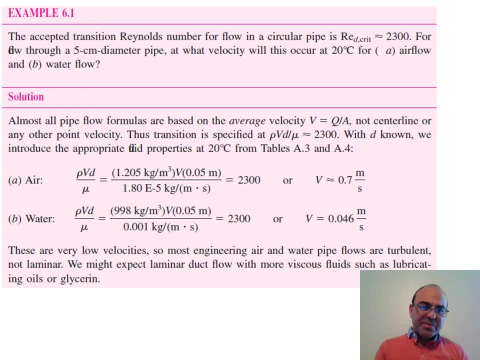 So, in this example. We want to see what is the range of the velocities to have. 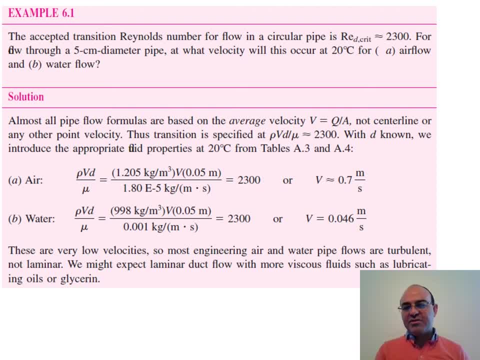 Laminar flow and. Turbulent flow. 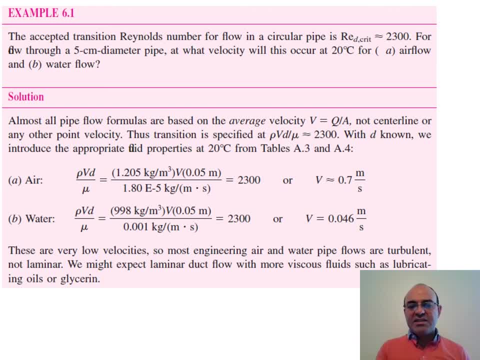 Or in other words. How high the velocity could be. 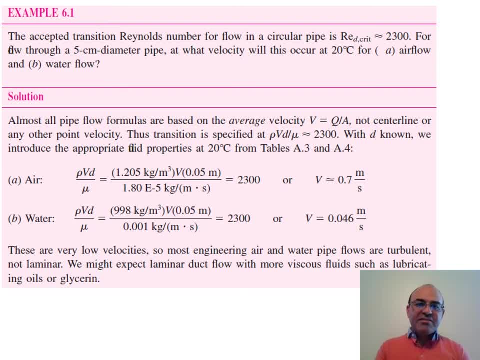 Before it becomes like turbulent. So, the accepted transition. Reynolds number for flow in a circular pipe. 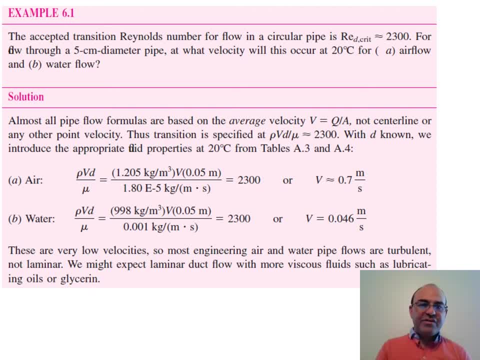 Is 2300. For flow through a 5 centimeter diameter pipe. At what velocity. Will this occur. At 20 degrees C. So, properties evaluated at 20 degrees C. 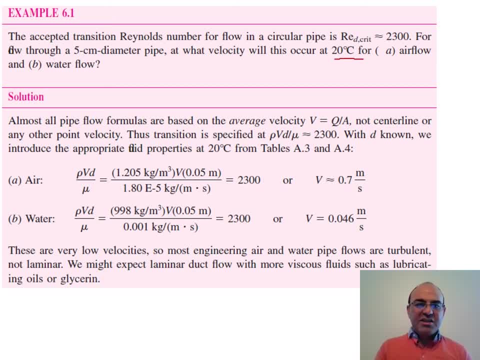 Density and viscosity. The tube diameter is given. And we want to see at what velocity. 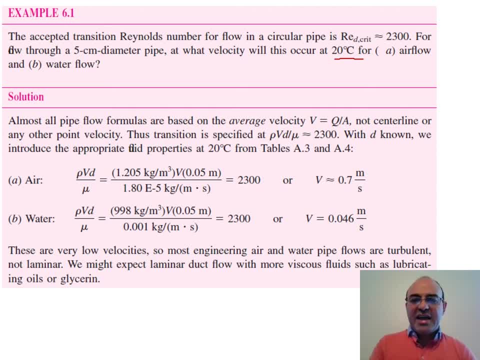 Transition from laminar to turbulent occurs. A for air flow. And B for water flow. Okay. 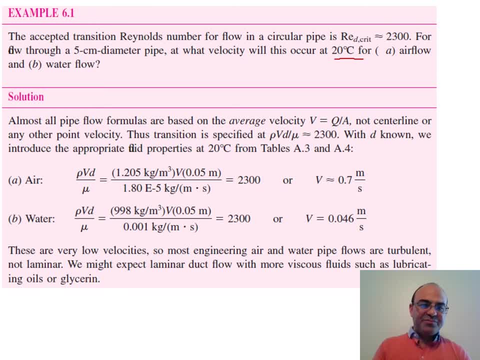 So, we use the definition of Reynolds number. And put it equal to 2300. Case A. For air. The density of air. Velocity unknown. Diameter 5 centimeter. 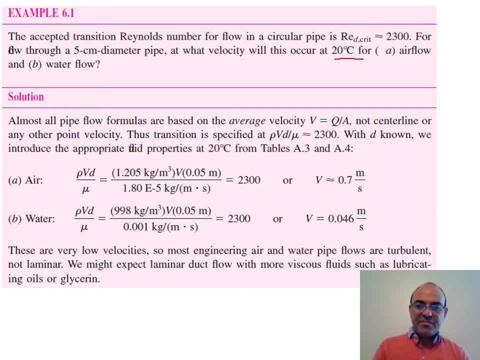 Viscosity of air. It turns out that the velocity. Is 0.7 meter per second. For air. 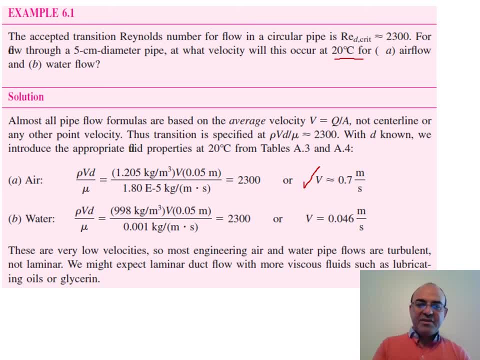 So, for similar thing for water. If we substitute the properties of water. Density of water. And same diameter. And unknown velocity. Viscosity of water as you see. Is much higher than viscosity of air. The dynamic viscosity of water. Is much higher than dynamic viscosity of air. 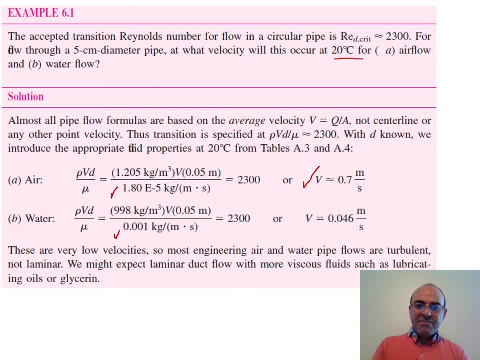 So, as a result. The velocity which. Makes the flow turbulent. 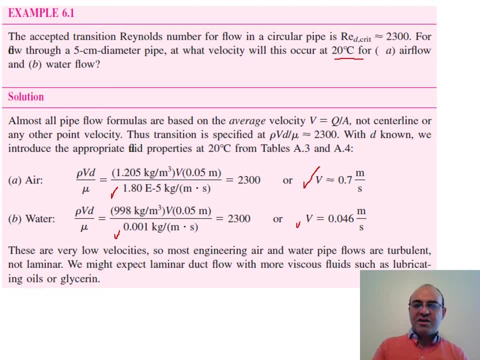 Is very small. In the case of water. In a tube of 5 centimeter diameter. So, 5 centimeter diameter is like. 2 inches. Right. 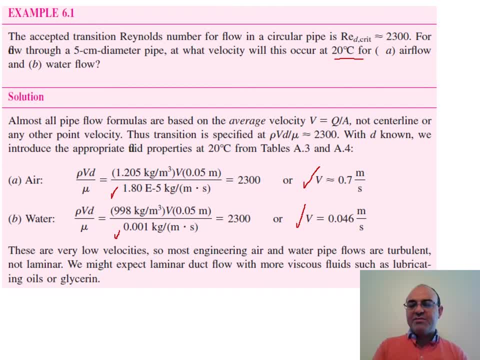 So, the flow is like about 5 centimeter per second. 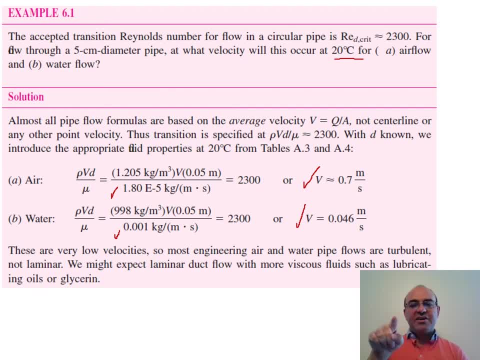 So, 5 centimeter per second. Is like it's a very small. 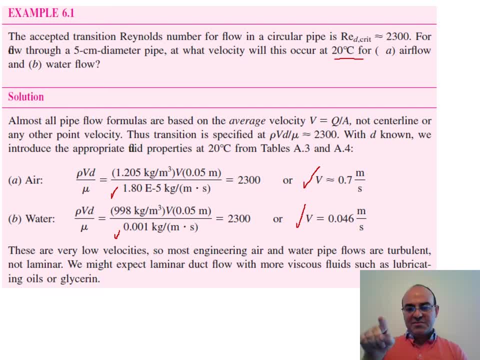 Low velocity flow is 5. Meter per second. 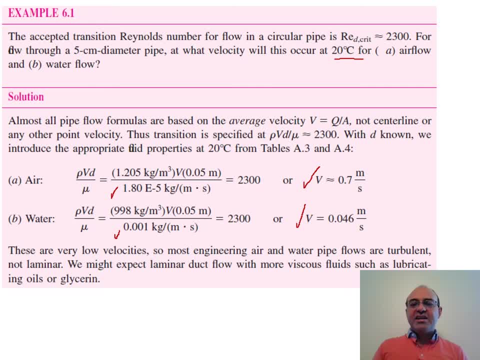 So, it is. The limit of laminar. So, in real cases. So, let me repeat. So, let me read through this discussion here. 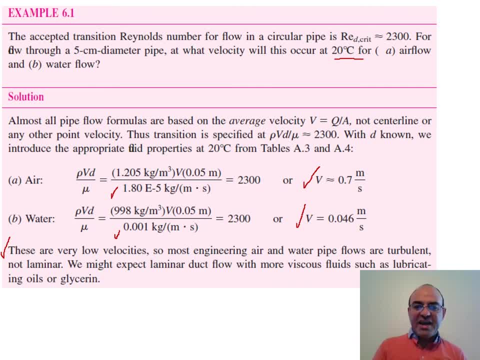 So, these are very low velocities. So, most engineering air and water pipe flows. Are turbulent. Because in reality. The velocities which are used. Are higher than these values here. So, not laminar. So, therefore laminar flow is kind of more. 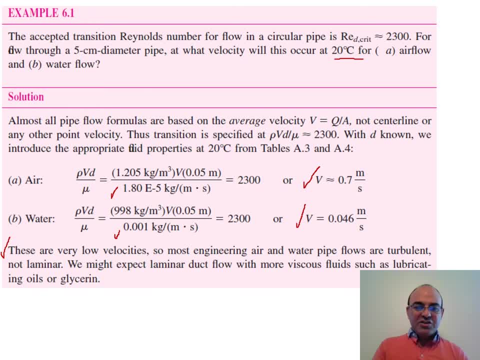 It's like it has more theoretical value. So, we might expect. 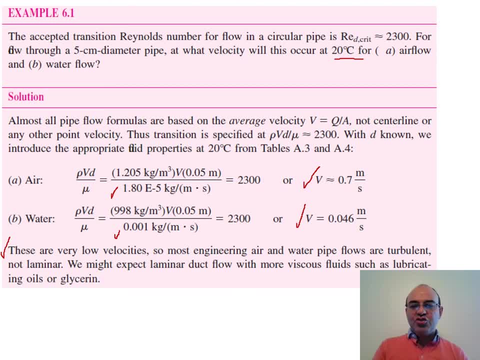 Like a It's like. 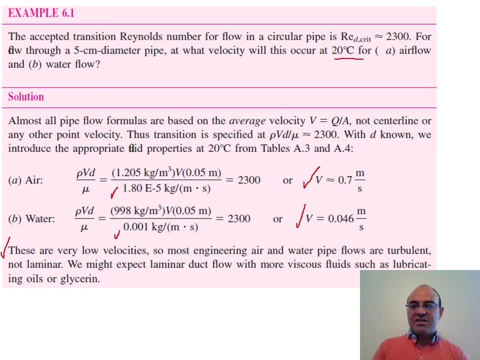 1. 2. 3. 4. change 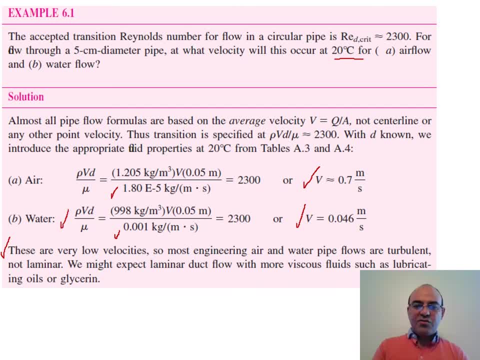 so for instance if you use oil in instead of water if you use oil then the viscosity becomes let's say 10 times larger even 100 times larger for like some oils or glycerin so then if the viscosity becomes larger for the same Reynolds number the velocity can become larger like 4 meter per second or 0.4 meter per second 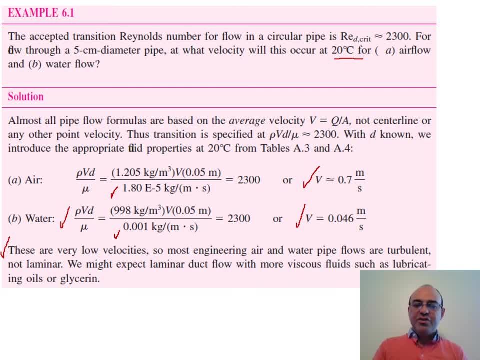 so in other words for a more viscous fluid such as oil the flow remains laminar within a broader range of velocities and that's something that you can imagine because oil is more viscous more sticky it is harder to make it turbulent 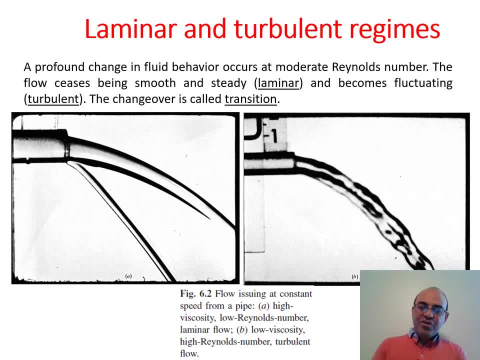 okay so here on the left you see a laminar flow you see that it is quite laminar so as the the name suggests laminar flow there is no turbulence no disturbance and if disturbances occur if for instance you like gently hit this pipe here you see like some vibration but it will damp away because it's a laminar flow a profound change in fluid behavior occurs at moderate Reynolds number so when it becomes transition and then turbulent the flow ceases being smooth and steady laminar and becomes fluctuating turbulent the change over time is going to be a little bit more complicated because the change over is called the transition so what you see 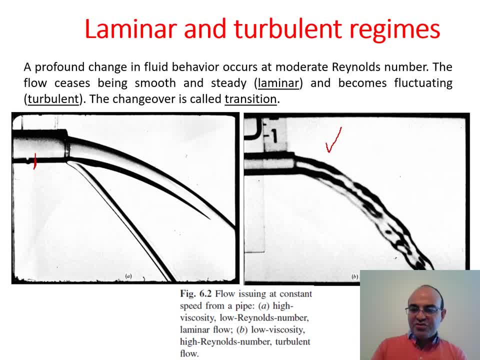 here on the right it's like a transition and turbulent flow 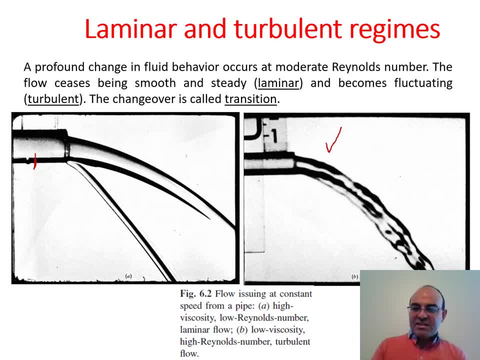 so you see that the surface of the this emergent jet is like wavy so you see the waves and disturbances and turbulence so this is like a turbulent flow on the right 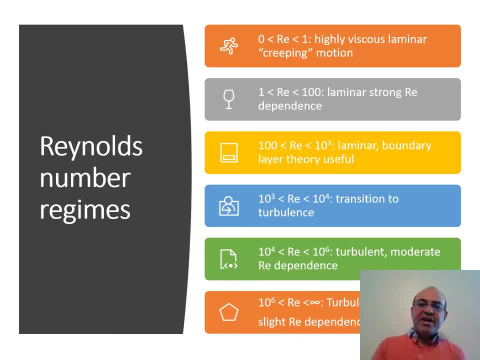 so if you want to see the range of the Raynor's number so if you want to see the range of the Raynor's number so if you want to see the range of the Raynor's number if you want to basically break it down to smaller ranges of Raynor's number so for very low Raynor's numbers between zero and one 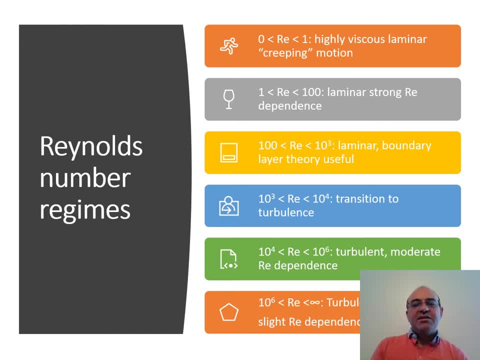 so it means that the the momentum the Reynolds number what is the Reynolds number is the ratio of inertia forces divided by the viscous forces so if Reynolds number is very small it means that the viscous force is very strong so if Reynolds number is very small it means that the viscous forces are very strong so this is therefore a highly viscous laminar flow which is called creeping flow creeping motion 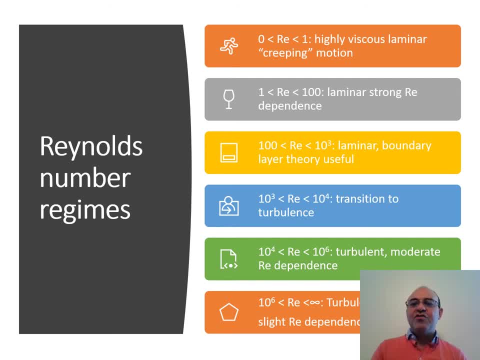 or stokes flow because it was developed by an engineer scientist engineer stokes 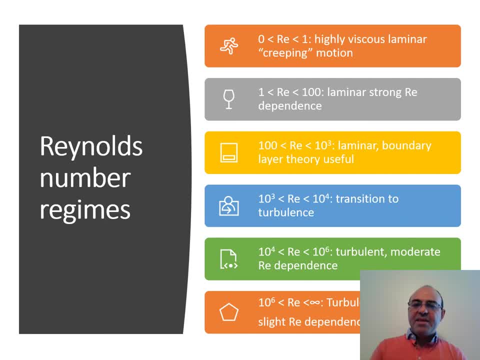 so as we increase the Raynor's number then between 1 and 100 it's like in a pipe this is still laminar flow but the but still there is a strong dependence on the Reinhardt's number. 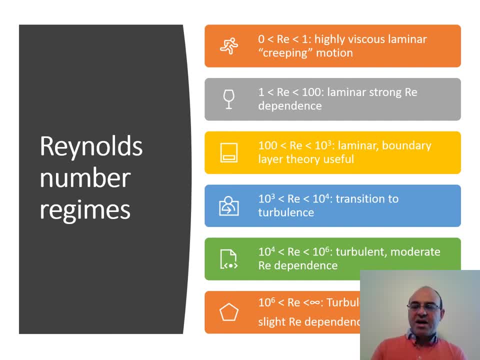 Between 100 and 1,000 in a pipe, it's still laminar flow. 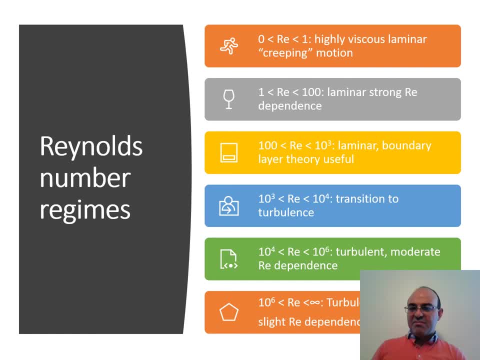 Boundary layer theory is useful. So we will talk about boundary layer theory a little bit in this chapter, 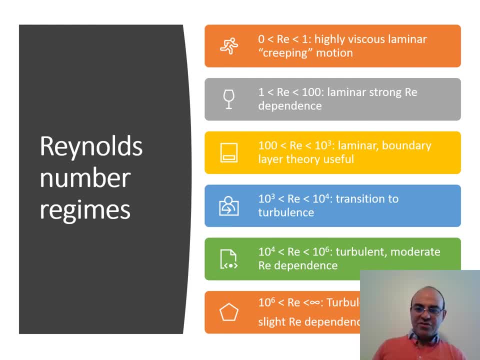 but mostly in the next chapter on external flows. 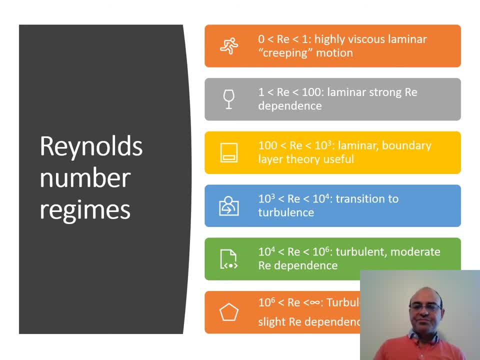 So basically a boundary layer is, so when we do have a fluid flow next to a solid wall, so that solid wall is called a boundary, but very close to the boundary, the viscous effects are important. Far from the boundary, the viscous effects become less significant. So the boundary layer. The boundary layer means the layer of fluid, which is under the effect of viscosity and it is very thin and it is close to the boundary or the walls, the walls of, for instance, the walls of the pipe. 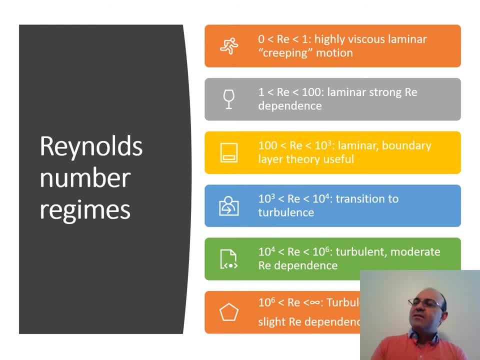 Then Reinhardt's number of 1,000 to 10,000. So 1,000 to 10,000, we know that 2,100 and 4,000 for laminar flow, fully turbulent, these are actually in this range. 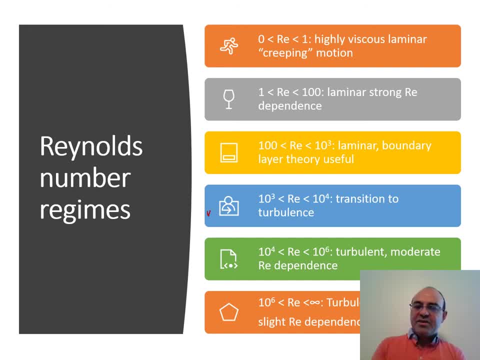 So this is the transition to turbulence range. 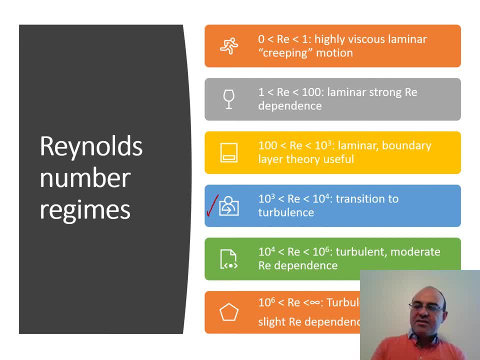 And for the Reinhardt's number higher than 10,000, it is definitely turbulent. Up until 10 to the sixth, we call it moderate Reinhardt's number dependence. It is turbulent flow. The dependence of Reinhardt's number is moderate in terms of like the, like effect of the pressure drop, friction factor, and so on, that we will see later. 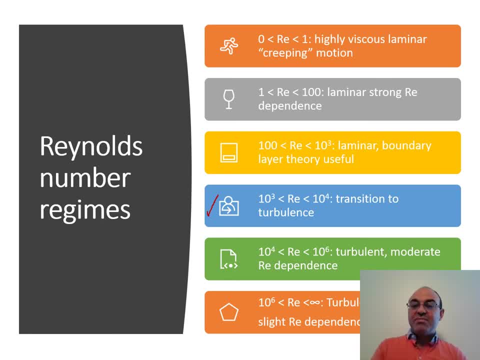 And Reinhardt's number is larger than 10 to the power of six. It is fully turbulent. I mean, it's already, it's been turbulent before. 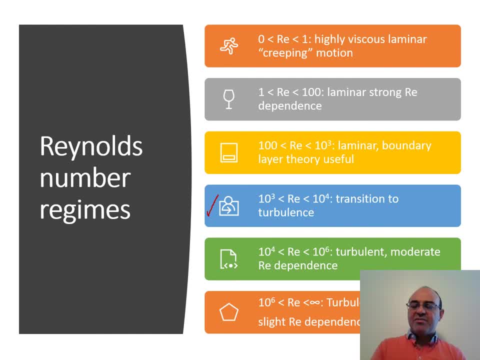 It's turbulent again. And the dependence on Reinhardt's number in the design conditions is negligible. 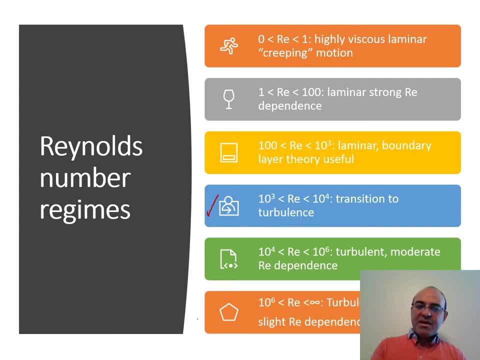 So we will see this. These things that you see here, we will see this later when we want to calculate the friction factor and the pressure drop in a pipe. 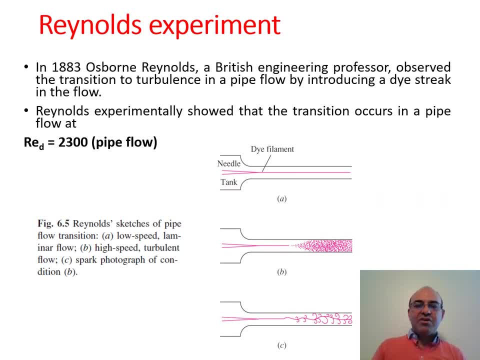 So in 1883, Osborne Reynolds, a British engineering professor, observed the transition to turbulence in a pipe flow by introducing a die strip. . 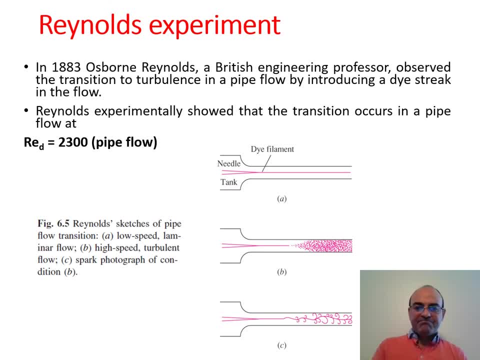 So, in the case of like, A, it's a low speed laminar flow, if you add some seed particles or like the die and then picture the process using like a transparent pipe, so like a glass or plexiglass or any kind of other transparent pipe, if you release a die, you see that it will move, it will not be dispersed. 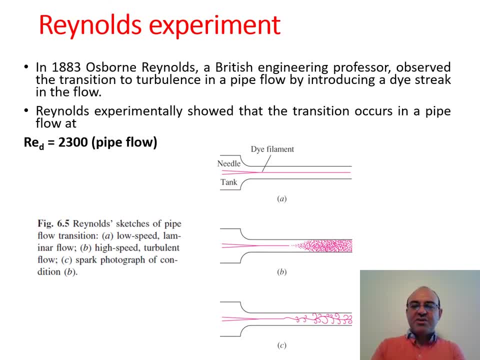 Let's put it this way, it will not be dispersed. So, that's the property of a laminar flow. 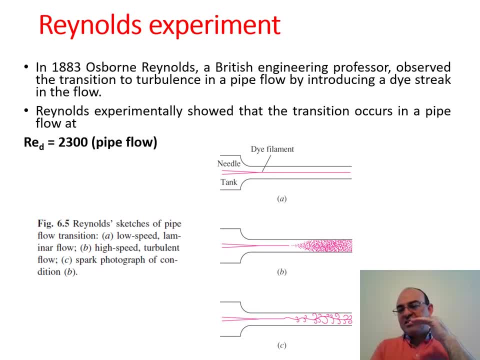 Because laminar flow is laminar, it does not, it's not, it doesn't disperse like the die. 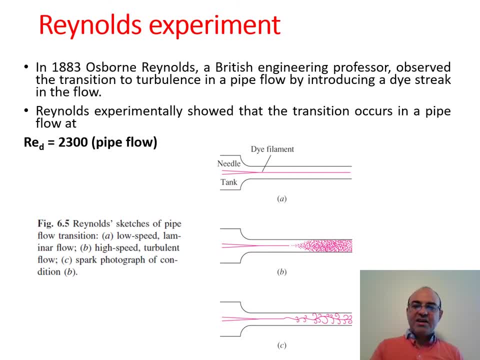 So, the streak line will be just like a straight line. This is also like the stream line and the path line. Now, if the flow is turbulent, a limit that he observed to be 2300 between like laminar, 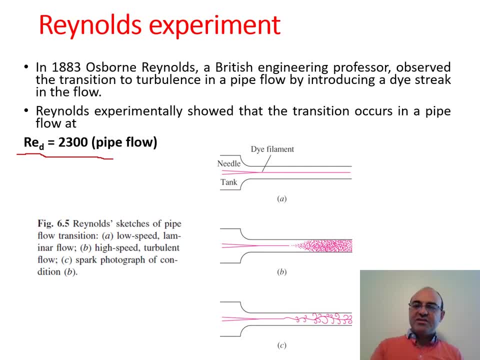 turbulent, 2300, and that's the limit that we use now, then he observed that the die would disperse and, you know, if you, if you take a picture, well, this is what we actually happen, this is a schematic of the turbulent flow. 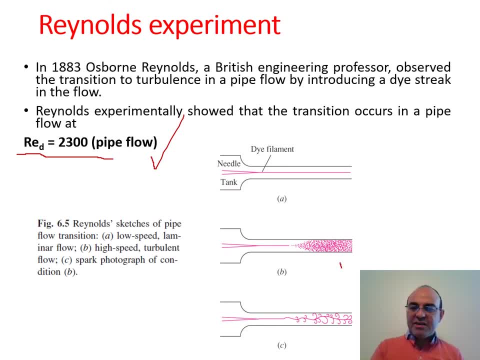 But if you take a picture of this turbulent flow in B, so if you take a picture using, at those times, using like a flashlight, a spark photograph of this condition, then he observed a situation like what you see here. 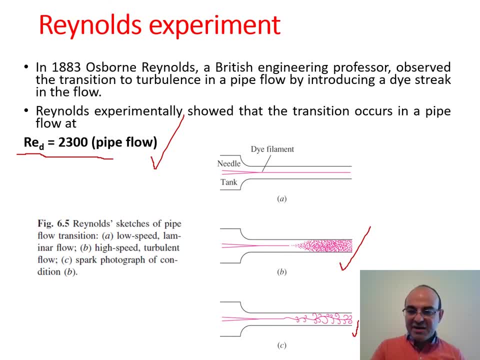 So, he was able to freeze some of the branches of the flow and the flow looked like this. So, C is like turbulent as seen in the pictures and A is laminar. 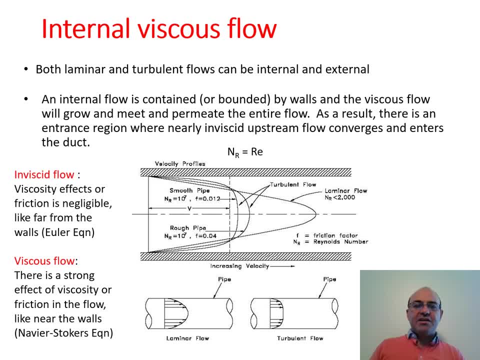 All right, so a flow, either viscous or inviscid, could be internal or external. Internal flow occurs, you know, in the case of flows in a pipe or in a duct. External flows are flows like over an object such as a sphere or, a wing or aircraft and so on. 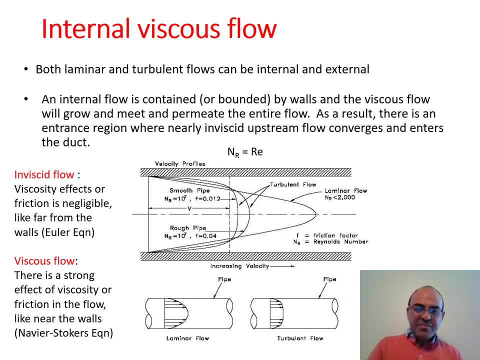 So, we can, we usually define two cases, cases, a case of inviscid flow and viscous flow. So, let's see what this, what it means. 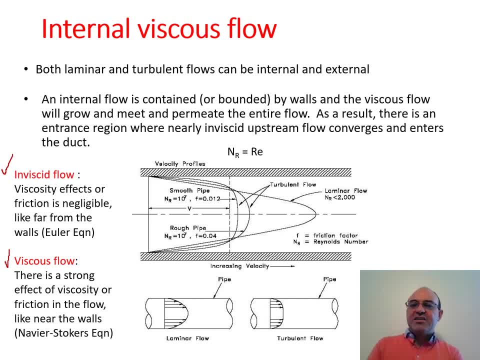 And we actually have had it in Chapter 4 as well when we talked about Euler equation and Navier-Stokes equation when we derived the full Navier-Stokes equation. 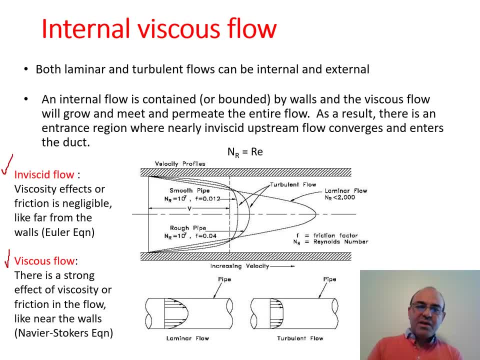 So, inviscid flow is a flow in which viscosity affects or friction is negligible, like flow far from the walls. So, in reality, viscosity is always present, friction is always present. However, if you do have, let's say, this is like a boundary, a wall, a plate, and you do have a flow next to the wall, you do have a boundary layer and a strong viscous effect. But further away from the boundary, the effect of the viscosity becomes negligible. So, it's like the effect of the viscosity is not sensed. Or it doesn't affect the equation. It does not create velocity gradient. So, if that's the case, the flow is called or considered as inviscid. 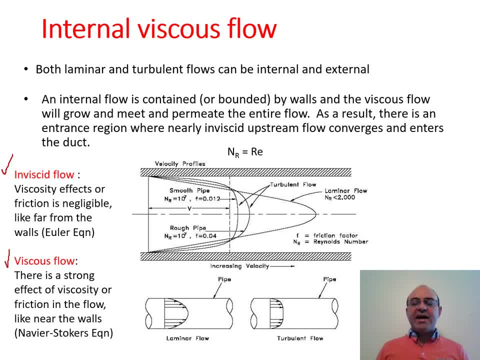 In this case, the analysis of the problem becomes much easier, and the Euler equation is the governing equation. So, basically, what is Euler equation? 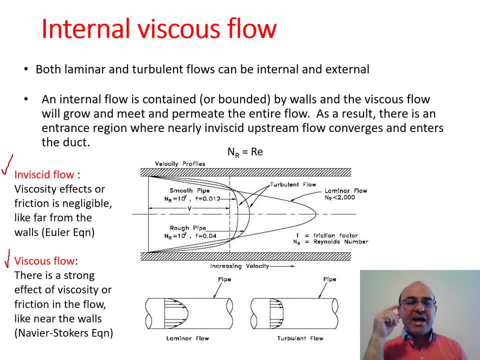 If you look at the Navier-Stokes equation and drop the term, which has... Viscosity in it, then you will actually establish the Euler equation. 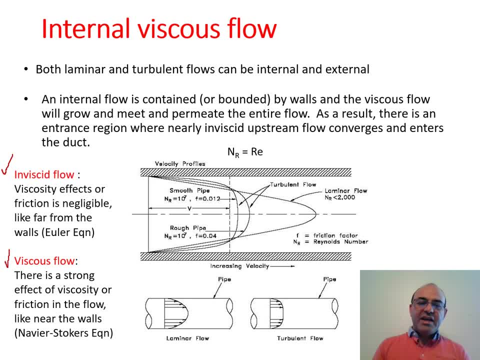 Viscous flow. In a viscous flow, there is a strong effect of viscosity or friction in the flow, like near the walls. 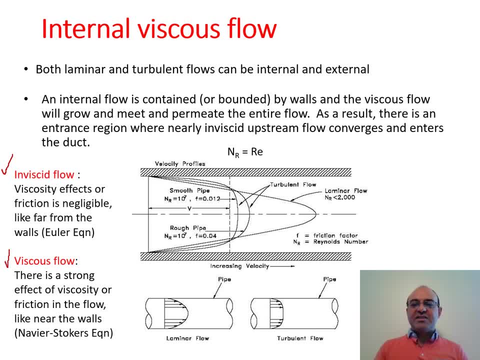 So, in this case, the full Navier-Stokes equation governs the flow. 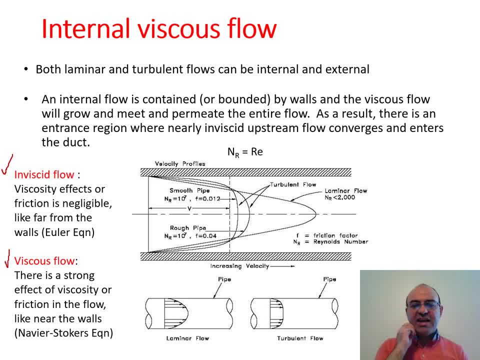 Now, if we look at the profile of the laminar and turbulent flow... in a pipe let's see how it looks like so first of all in this diagram NR is the 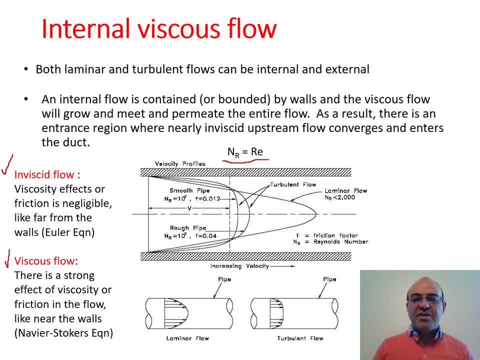 same as Reynolds number so in some books Reynolds number is shown as NR means the Reynolds number or number associated with the Reynolds number so we know that in the case of a laminar flow the velocity profile is parabolic so what you see here it is probably is a little bit of stretch this this is not this probably shows the parabolic velocity profile in a better way from previous chapter as the fluid becomes turbulent because of the mixing effect the fluid 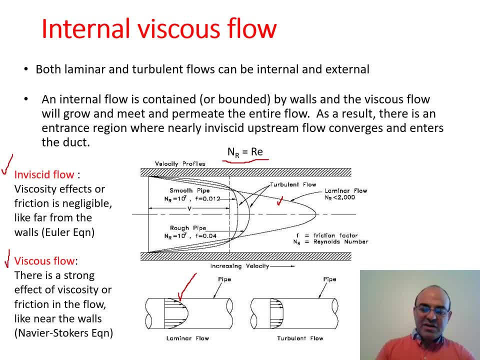 profile becomes more uniform so therefore in a unit in a turbulent flow the velocity become profile becomes kind of uniform as you see here as the Reynolds number increases it becomes more uniform or flat so therefore here is the laminar flow and then these two you 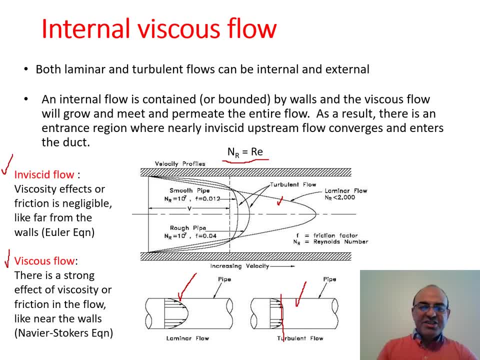 okay so there is an entrance region very nearly inviscid upstream flow converges and inter enters the duct so here we talked about inviscid flow and viscous flow and that's related to the entrance region that we will talk about in the next slide in more details 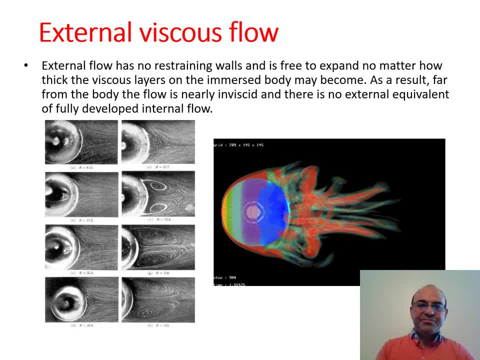 so we talked about internal flow and we said that some of the other flows are external the topic of the next chapter so external flow has no restraining walls and is free to expand no matter how thick the viscous layers on the immersed body may become so this is for instance on the right side you see a sphere and then very closely very close to the surface of the sphere we do have the 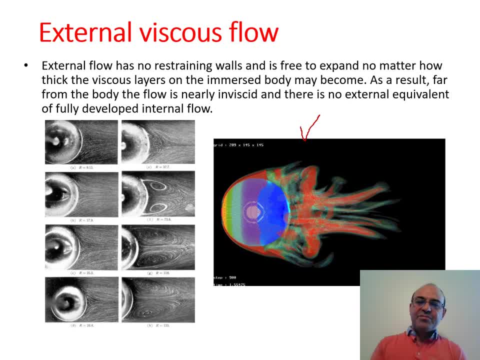 boundary layer where the effect on viscosity is very strong at the back of it it's like circulation is called a wake pressure drop and turbulence we 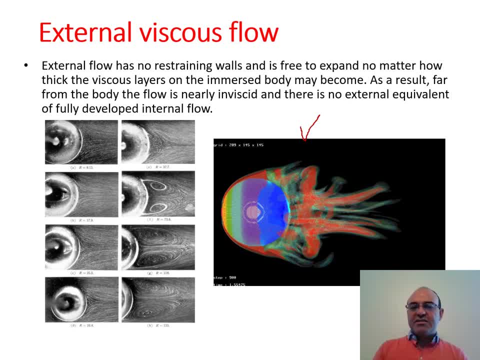 will see it in the next chapter so this is the this is an example of it of an external flow what you see in this on the left is the surface so it is a particular flow of the flow displacing孩子 this on the left is起源 flowing to the top the surface we will see it by ouruz 然後 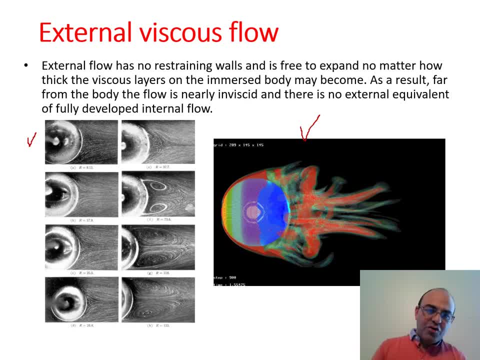 is flow over a sphere or like a cross-section of a cylinder and it is very small but Raynor's number increases so at the left the first picture this one Raynor's number is very small 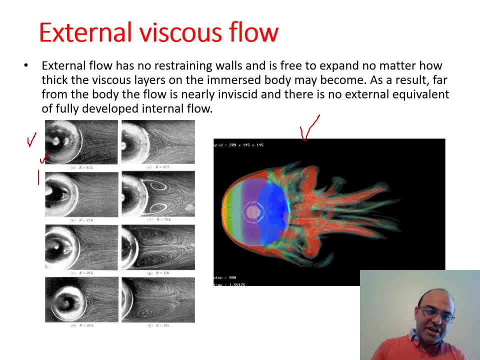 and from top to bottom the Raynor's number increases so you see that the Raynor's number increases but it is still laminar the Raynor's number is still small and then on the right side we keep increasing the Raynor's number and then you see that at the back or downstream uh of the this sphere you see that circulations start to form you do see circularity start to form and then you see that the circulation starts to form and then you see 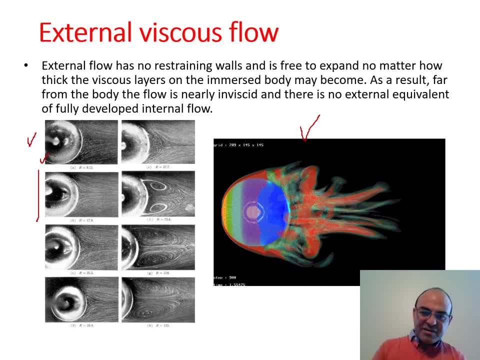 some separations from the boundary from the surface of the sphere and so development of like circulations here and you also see them here so that's the 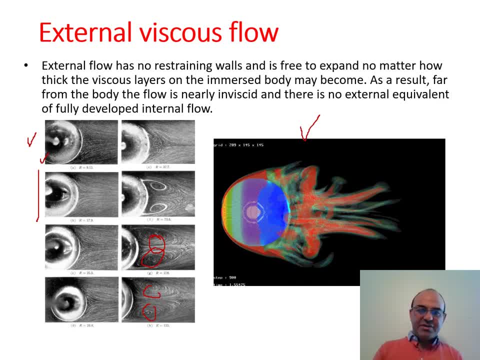 external flow that we will talk about in the next chapter you 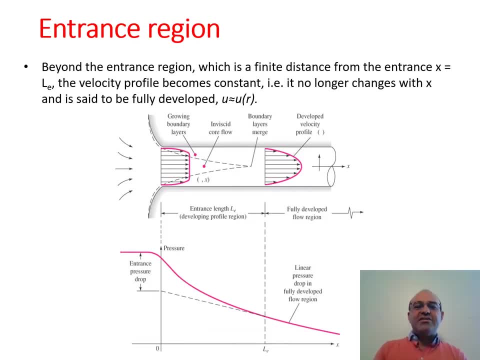 so now what is the entrance region that we talked about a little bit in the previous slides so let's say you do have a duct or a pipe what you see is like a pipe and then this is the entrance on the left side you see the entrance of the pipe so as the fluid from the upstream is coming in it is it comes in like with a kind of so that it's it does have a uniform velocity this velocity profile it comes in so as soon as it comes in the fluid close to the surface or close to the boundaries or walls of this tube will be influenced and will be affected therefore a boundary layer forms right next to the walls and you see this dashed line that's the boundary layer or that's the edge of the boundary layer this figure is not to scale so the boundary layer thickness is much smaller and it takes a longer time for the boundary layers from all sides of the wall to actually merge so after some time you see that the 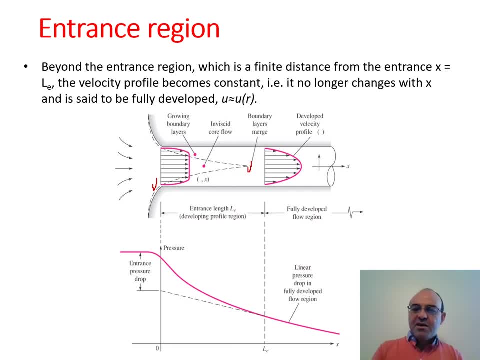 boundary layers will actually merge so but so there is therefore a development in the system to allow the boundary layers to merge and this is what we do here is to be able to show how the boundary layers merge so in the middle or in the centerline of the pipe the velocity remains uniform or remains the same as the velocity of the upstream here and there on the surface of course the velocity is zero and then it can it starts to change its shape and then it to grow so we do have a velocity profile like this at the entrance so at the center uniform velocity on the surface zero and then there is a sharp or a steep gradient of velocity to connect the surface the surface velocity to the center velocity so once it is fully developed for the laminar flow we know that the fluid profile becomes parabolic so that's the parabolic flow profile and after this point this profile does not change anymore so it remains unchanged because the velocity profile if you remember is only a function of r the radius so the radius measured with respect to the center line and it is not the function of x so it 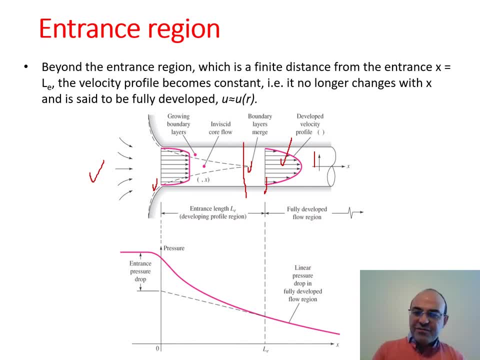 doesn't change with x so after this point the flow is called fully developed so this is fully developed flow region so it is it starts once the boundary layers from all sides well a round tube doesn't have a side from all points of the wall actually 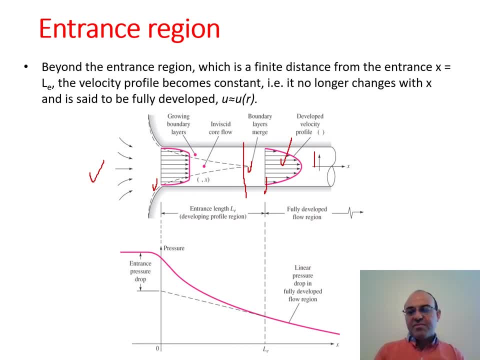 merge and then they create a parabolic velocity profile before that that's called the entrance region or the developing region developing flow region or entrance region so on the left here we do have developing or entrance and on the right of this line we do have the fully defend and 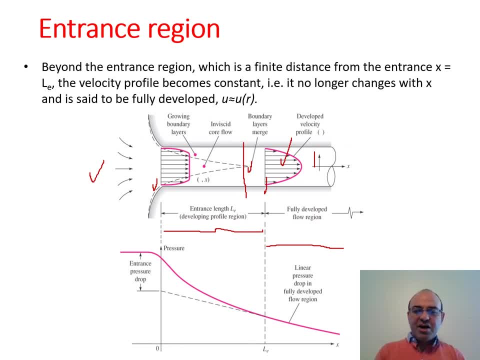 the behavior after fluidity and if you want to say different between them you can measure the flow such as the pressure drop is different in the fully developed and in the developing region so sometimes it is important to have an estimate of the 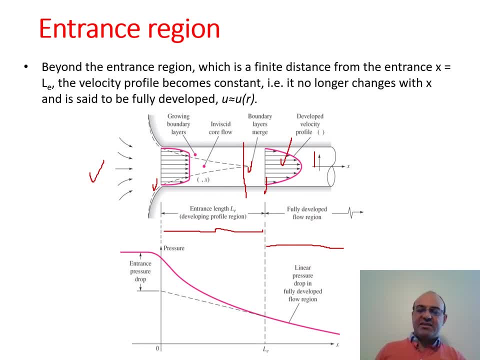 entrance length but often time we neglect it so we will see it in the next slides 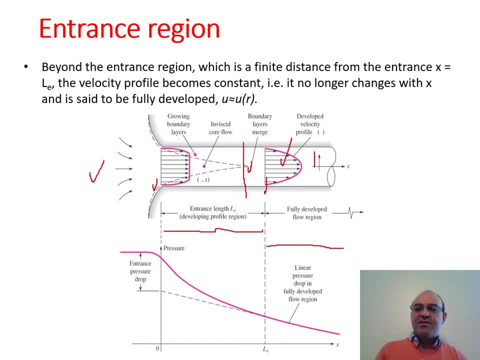 how we want to actually calculate or estimate the length of the entrance region to see that if we do have a laminar flow after what distance from the the inlet we can actually assume that the velocity profile is like a 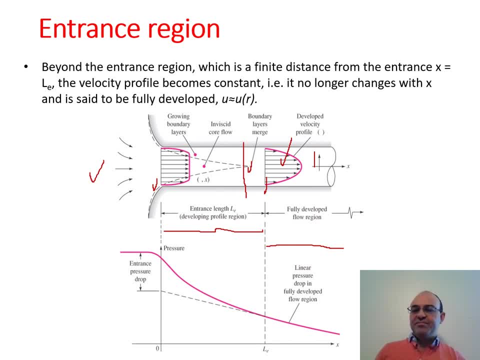 parabolic in the case of a laminar flow 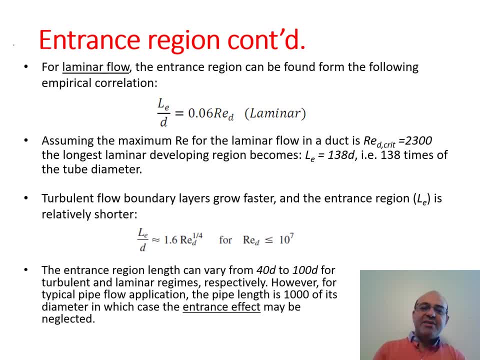 so the entrance region can be estimated using these equations so without going you know to the details of you know how to obtain it for laminar flow the entrance region can be found from the following empirical correlation so this is actually empirical it's been obtained by performing many experiments so the ratio of the L e the length of the entrance region divided by the radius divided by the diameter of the pipe is equal to 0.06 times Reynolds number with respect to the diameter of the pipe so that's for the laminar flow so assuming the maximum Reynolds number for the laminar flow like 2300 the longest it means that if you if you plug in the 2300 here in this equation then the L e becomes 138 times the diameter or in other words this value will become hundred three eight so it means that for a laminar flow if you have a laminar flow in a pipe with a diameter diameter one let's say one inch one inch diameter tube you 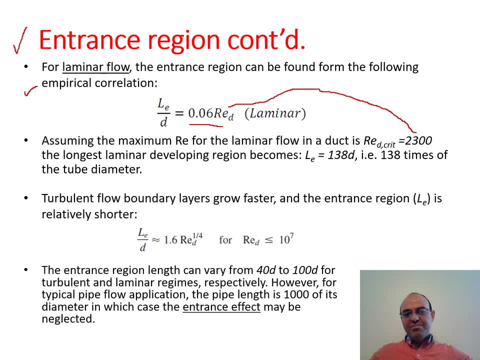 1 38 inches of the pipe will be in the developing or entrance region so this יכול быть 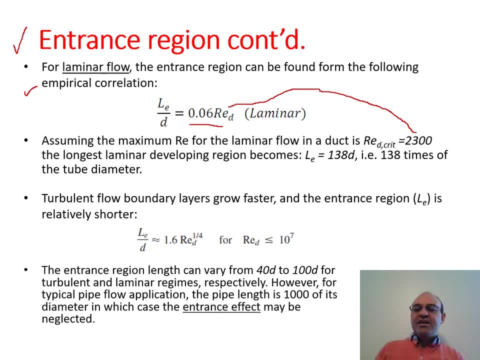 this can be quite long if your tube if the length of your tube if your tube is actually small so this can be quite large and therefore the entrance region 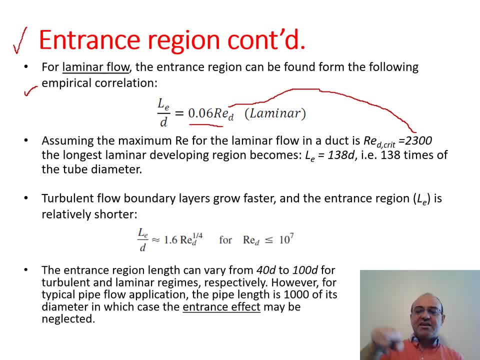 can be quite important however if you do have a closed circuit or the length of very large like it's a pipeline then this entrance length can be negligible compared to the rest of the length of the system or if you have like a closed system with a pump in it essentially you know you do not have to worry about the entrance region because the flow keeps circulating 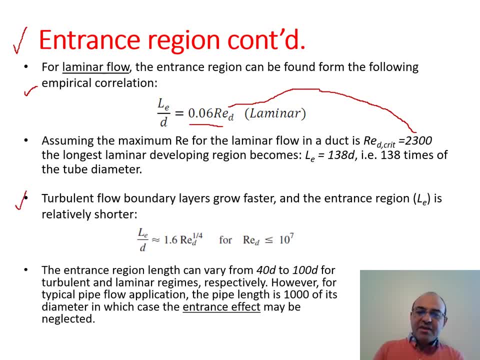 in the case of a turbulent flow the entrance length is obtained from this equation so L over D when multiple equations have been proposed this is one popular is this one is popular so 1.6 Reynolds to the power of 1 4th and this is good or best or works best and most accurate for Reynolds less than 10 to the power of 7 so 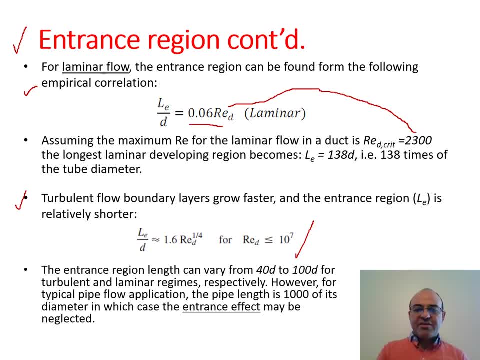 so as I said the entrance regions may be important in some cases but often time in fluid mechanics problems we neglect it because of the reasons that I talked about but if in a particular problem you do have a short tube for a particular application open circuit short tube fluid comes in and then goes out then the entrance region must be taken into consideration 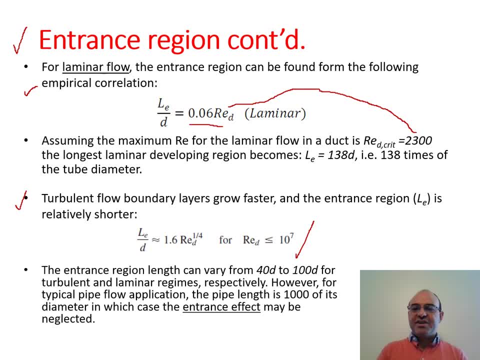 when you want to for instance calculate the pressure drop the friction factor and so on 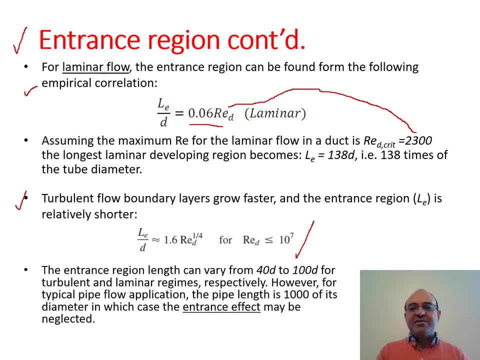 so what we will see in the rest of this chapter is actually for fully developed flows and not for the entrance region for entrance region some other equations and correlations are used which are kind of special cases and not covered so as an example here 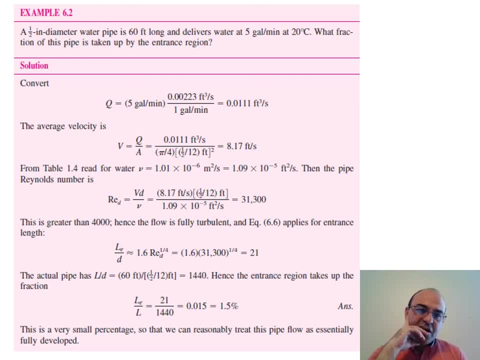 we have a pipe right here and the flow is very similar to normal so a pipe so we do have a diameter tube with given diameter fluid is water the length of the pipe is given 60 feet the units are not I units these are English units but we just go over the how to do the problem rather than looking at the numbers so we do have a pipe with given diameter and length and 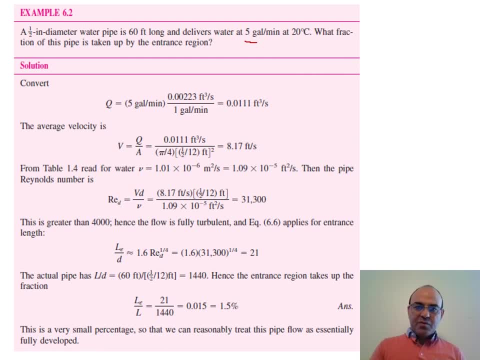 rate is given we want to see what fraction of this pipe is taken up by the entrance region so we want to estimate the entrance region and see that what is the length of the entrance region compared to the entire length of the tube which is 60 feet in this case so first of all in order to evaluate the length of the entrance region we need to know whether the flow is laminar or turbulent because for these two different flows we do have different equations to estimate the entrance length so first we calculate the velocity from the flow rate so the velocity is known then we calculate the Reynolds number Reynolds in terms of diameter Vd over nu Vd over nu so this is the same as rho Vd over mu but sometimes we instead of writing rho and mu we just use nu and nu is equal to mu over rho the kinematic viscosity so in this case it is 31,000 so we do have a turbulent flow then we go ahead and use the second equation in the previous slide L over this 1.6 times Reynolds to the power of 1 4th and this becomes 21 so LE the length of the entrance 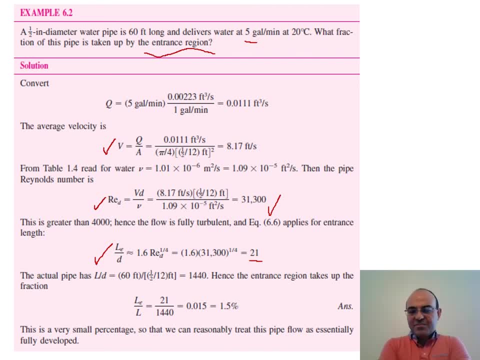 region divided by the diameter is 21 so since the diameter is known we can go ahead and calculate the actual pipe diameter the actual length of the pipe divided by its diameter is 21. 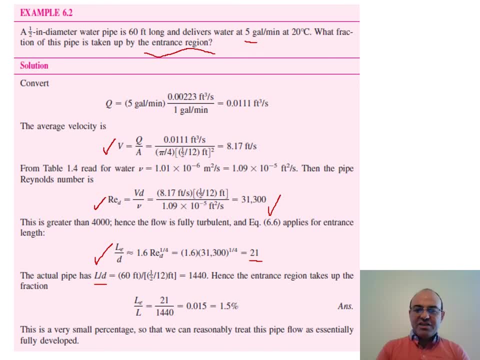 so the actual length over D is 60 feet or half an inch which is 1440 so you see that the entrance length with respect to the diameter is 21 the total length is 1440 so the entrance length is only 1.5.5. ..0.7.0.s. 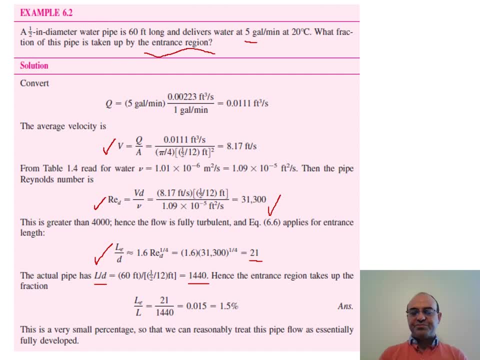 five percent of the entire length of the tube so this 60 feet tube or pipe